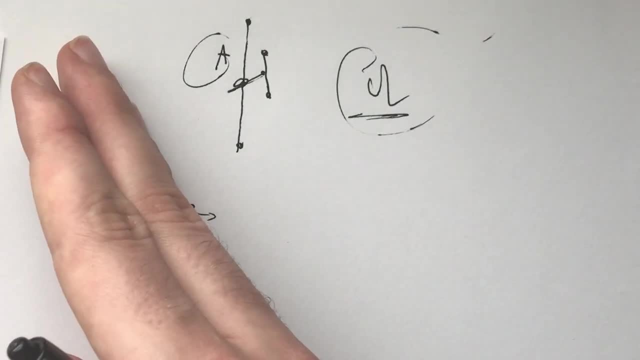 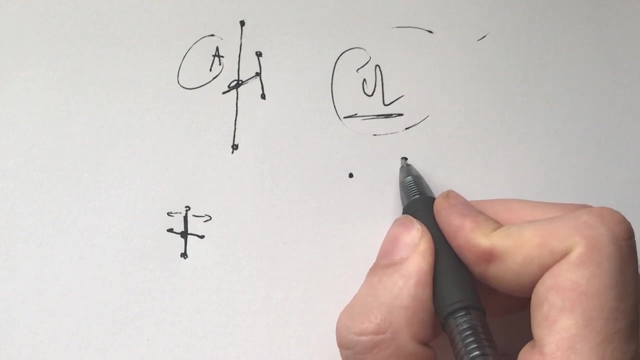 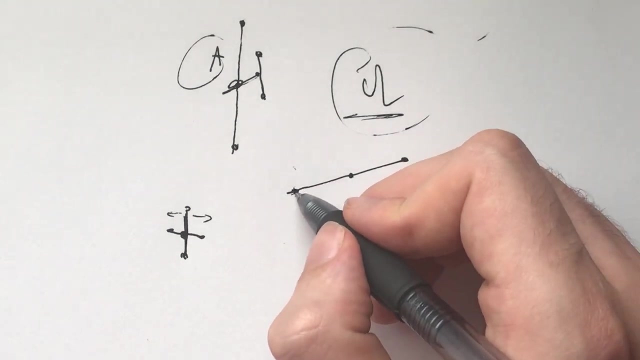 I can pick some points somewhere that's like the final point, And then maybe there's a point behind it, And how does that finality look like? Or you could also say: well, let me try to say: okay, what does it mean? Like, yeah, a midpoint between two points, And then I have another two, And this is again a midpoint. Like, okay, like could there be, is there some? 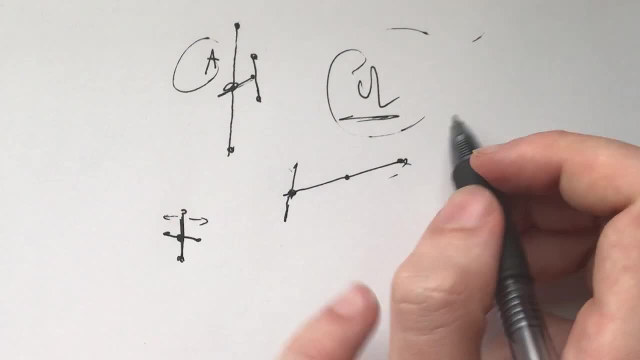 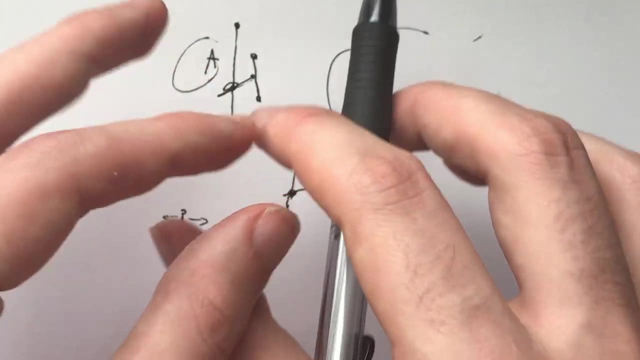 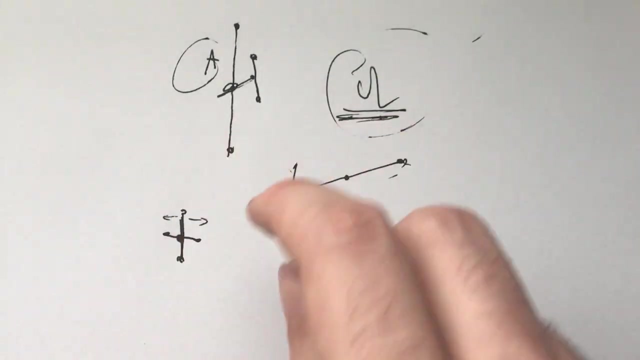 line property or some two points somewhere that make this infinite. that also has some sort of shrinkage or expansion property? And if they do, assuming the set is finite, what would you do with that? Take three to five minutes and try to think about these approaches, really Okay. so the first approach is again: assume the contrary in both approaches and take the points That's like further left. 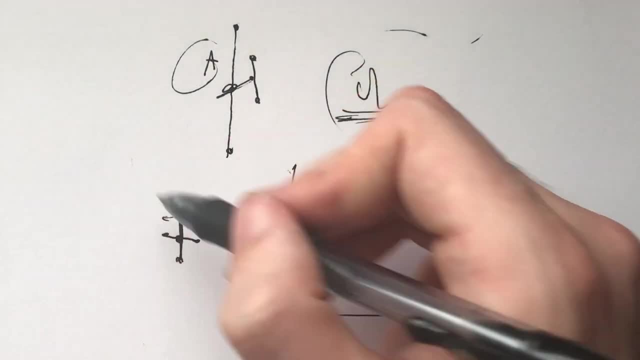 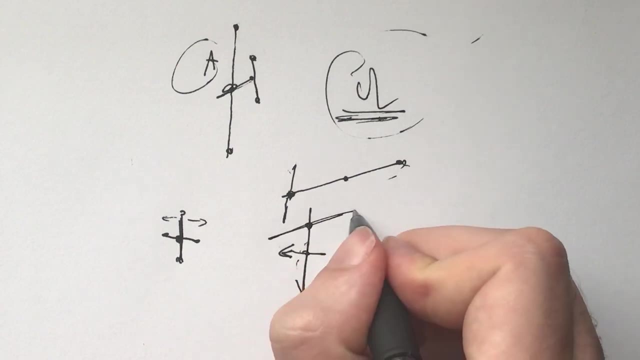 and if there's many points that are furthest left, like, take this left line, take the one that's furthest to the down, Why, When you take the one furthest to the left, now this can be a midpoint of some point that's more to the left, Like it can be if it's, if this point is M, it can be a midpoint of A- B, such that A is to the left of M because it's the most leftmost point. If you define left, you just draw these lines until you reach the final point, or final. 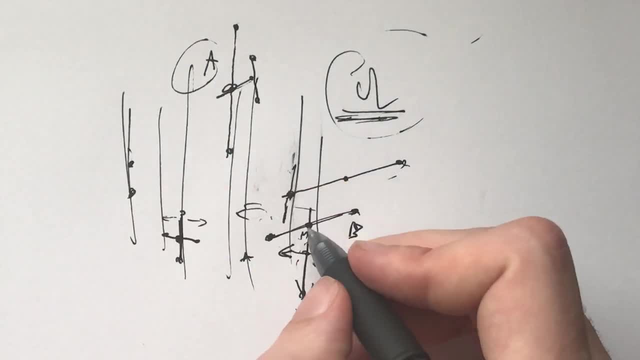 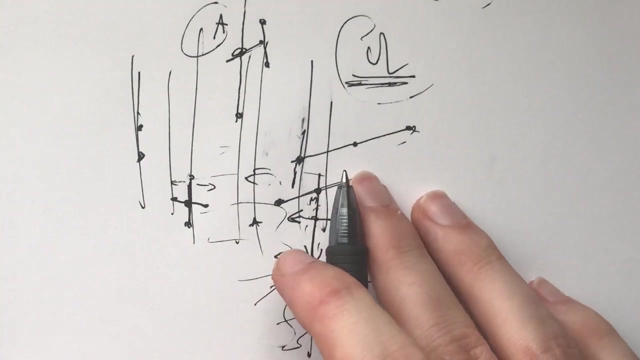 number of points and call this the leftmost point. Okay, so that's one thing, but there could be many points here, so you take the one that's in the corner, so there's no point that's below it or to the left of it. So all of this space- actually no more, like all of this space, including this line- is done. There could be other points here. And now, with that, what do you have? You have if this point, so there's no point that.